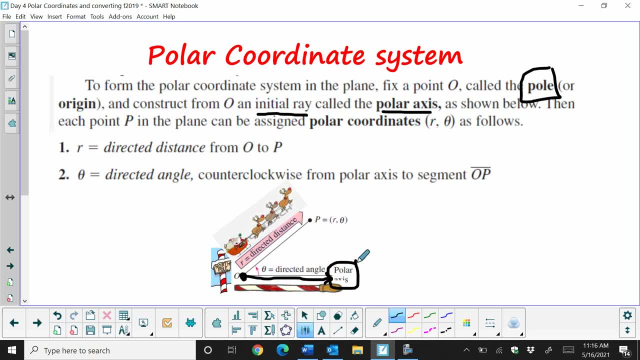 But in a polar system we call that the polar axis, And each point in the plane can be assigned a polar coordinate. And that coordinate is not an x and a y value, but an R and a theta value, R representing the directed distance which we've. 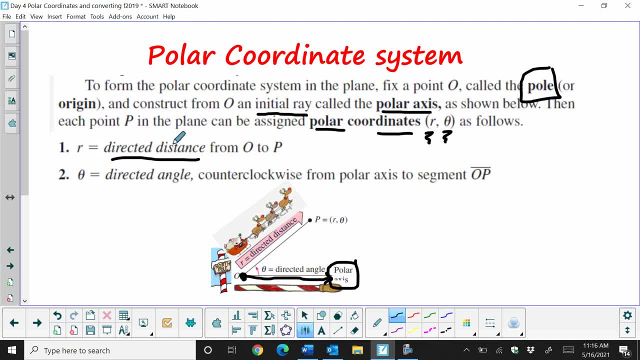 just worked on vectors. So that's just basically the magnitude or the length from O, the pole, to P, the end of that point, and theta. And theta is your directed angle of rotation And we always go counterclockwise, just like we. 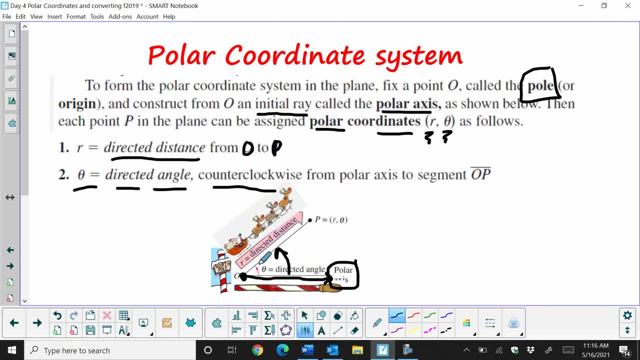 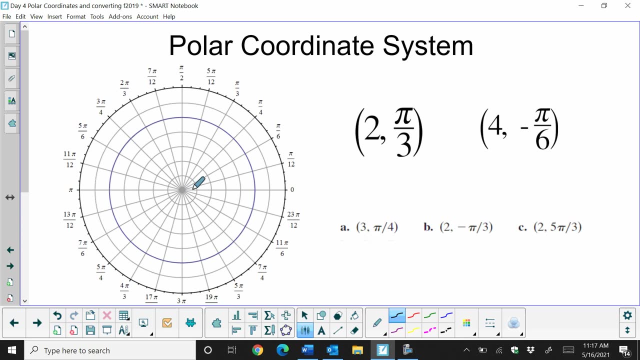 normally do on a unit circle. So you've got two pieces of the puzzle. You've got the length, which is R, and the rotational angle, which is theta. Now let's try to graph a few so you can see how this system works. We're going to start with the point 2, pi thirds. 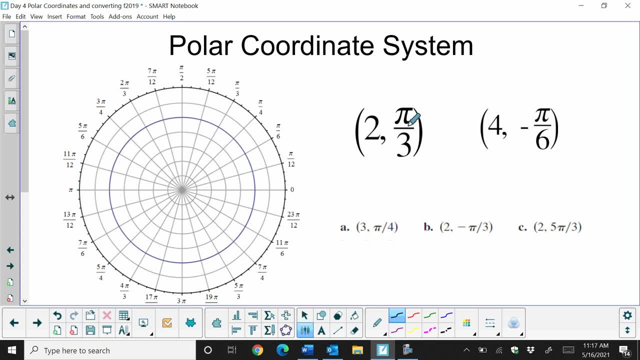 So notice 2, that's going to be my radius And pi thirds is going to be my rotation. So I'm going to start on this polar axis and I'm going to come out two units, which is to the second ring, And then I'm going to rotate around that axis to pi thirds, And that is the point we're. 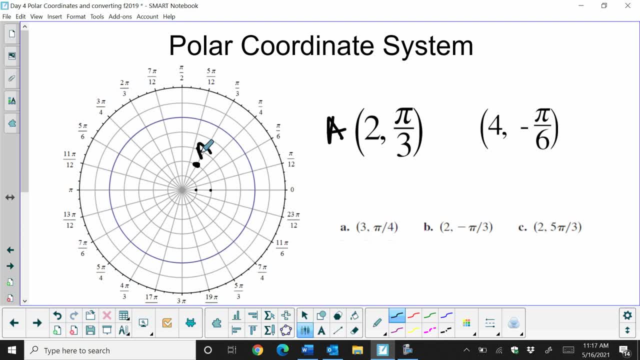 going to call that point A, Okay, and let's do the same thing with the second. So we've got the radius of 4, but this time we have a negative rotation. So that's going to look like this: We're going to come out 1,, 2,, 3, to the fourth ring or the fourth circle, But this time 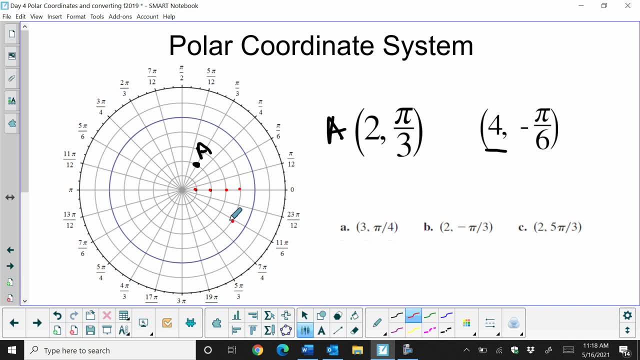 we're going to rotate negative pi sixths, And that puts us right here. Now, one thing I didn't point out is, on this polar axis, or on the pole, you can notice that our increments are in the pi twelfths. So when we're moving negative pi sixths, it's actually two twelfths. So that's why. 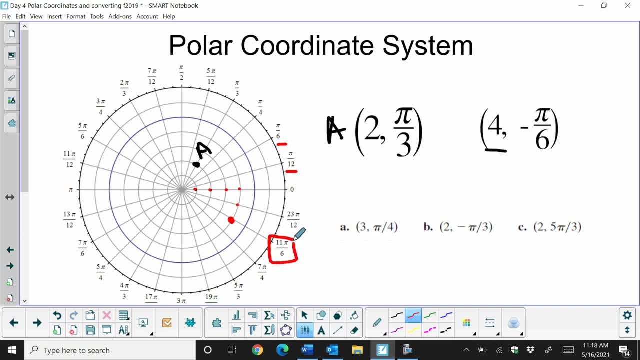 we went to the second position, which we also know as 11 pi sixths is negative pi sixths. So anytime you're rotating a negative direction, you'll go clockwise. Anytime you're rotating a positive direction, you're going to go counterclockwise, just like we've done with 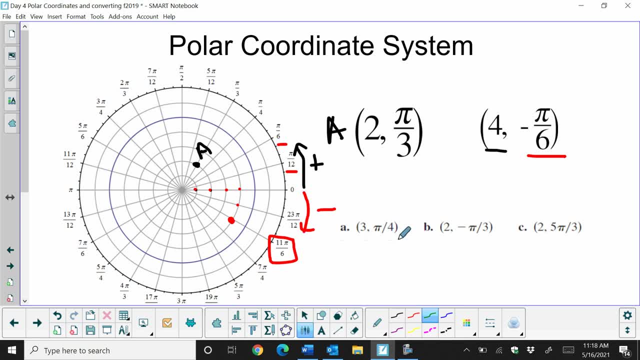 the unit circle. So now we have three more points to practice, So you can do this with me. This is 1,, 2, 3.. Go to the third ring And then we're going to rotate to pi fourths. So we're going to call that position. Let's call that C. 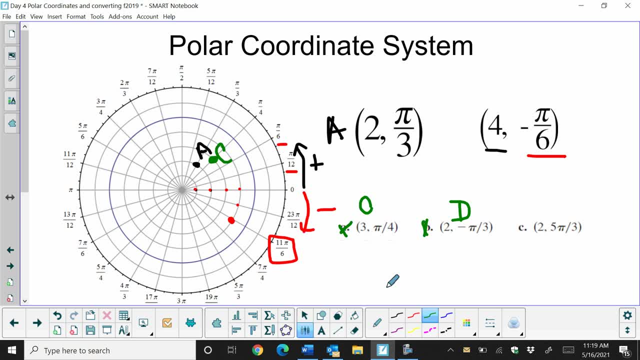 And let's try this one. This will be D And this is going to be 2.. So come out to the second one. This time we're rotating negative pi, third. So that's going to bring us to here And we're going to call that D. And the last one, we're 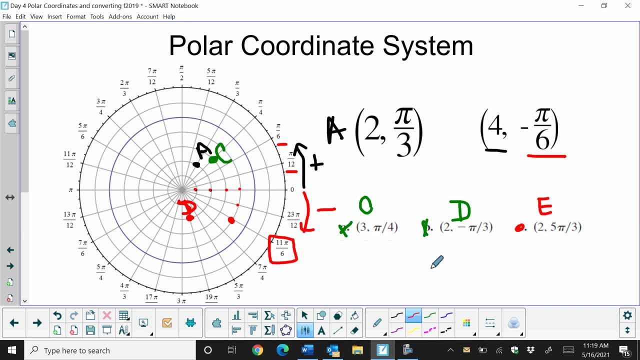 going to rotate in the positive direction, but this time quite a bit further. We're going to start on the second ring And then we're going to rotate all the way around to 5 pi thirds, And that puts us right here. It's the same position as D, So we can get to that position two different ways, And that's what we're. 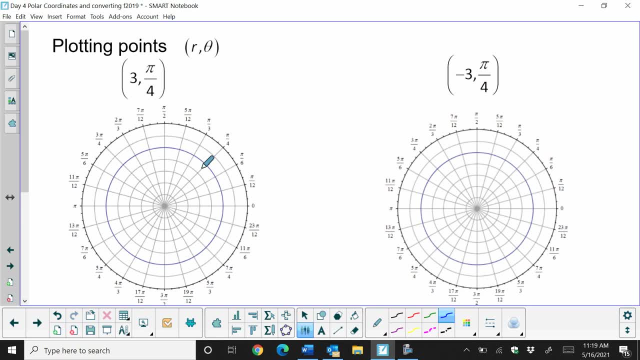 going to talk about next. Okay, Plotting points. Let's practice a couple more with positive radius and a positive rotation. So we're going to move this one out three and up to pi fourths. So here's this point And we'll call that X. 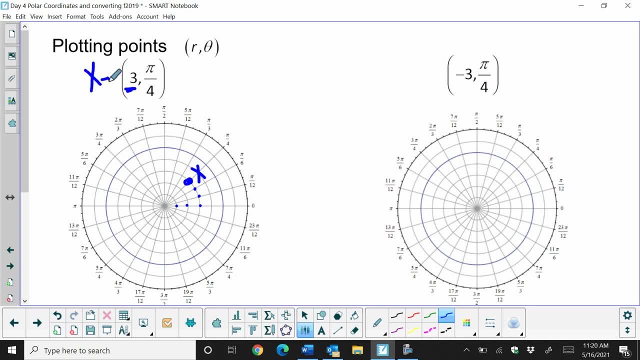 This is going to be our X. Okay, And we'll call this one Y. Now, this time I'm throwing something different at you. We have a negative radius, So instead of moving to the right along the pole, we're going to move to the left. So this one's going to start: 1,, 2, 3 in the negative direction. 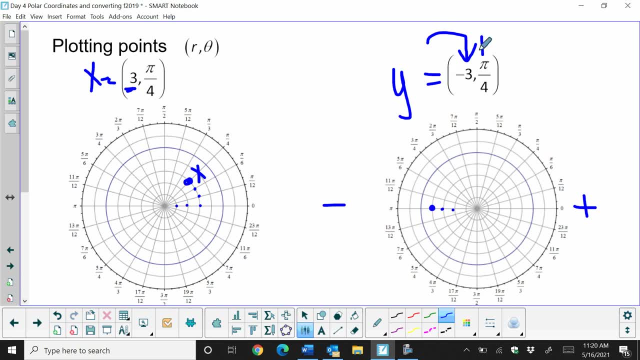 negative pole, But we're going to rotate pi fourths. Well, we know, when we're rotating in a positive direction, we're going to move counterclockwise. So that's going to put us right here And I'm going to call that Y. So I'm going to erase that, because this was just 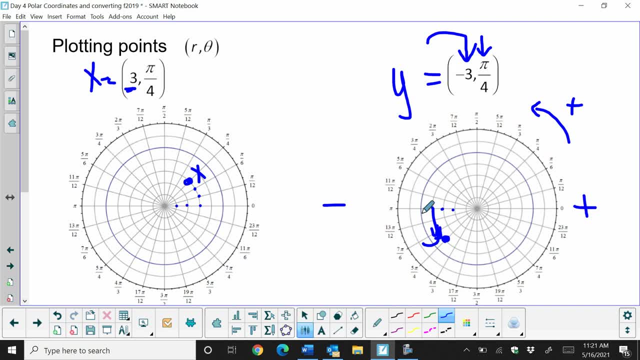 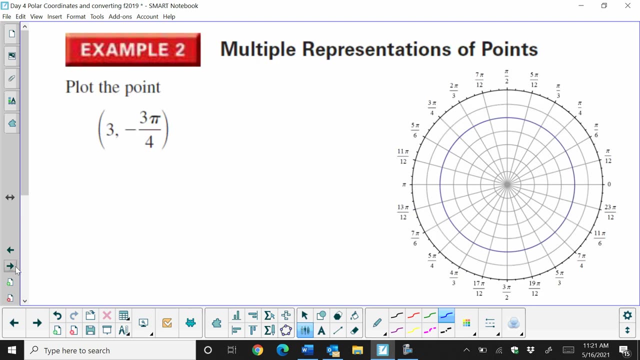 counting- That's not the point itself- And notice that rotation is pi fourths from that negative three axis. Okay, So we actually have different ways we can plot or we have different ways to name points when we're plotting in the polar system. So we're going to take the point 3, negative 3 pi fourths, And we're. 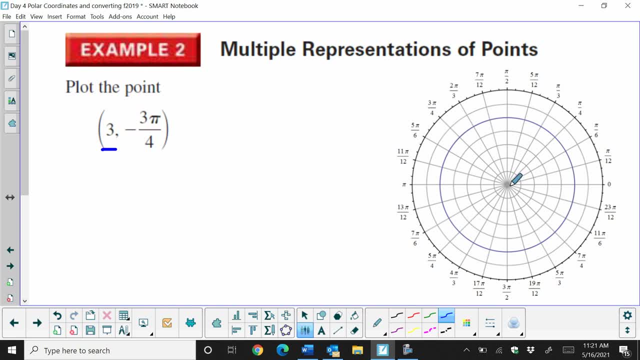 going to look at the different ways to write that point. So let's first just locate it. So we're at 1, 2.. We're on the third circle. We're going to rotate: 1 fourth, 2 fourths, 3 pi fourths. So there. 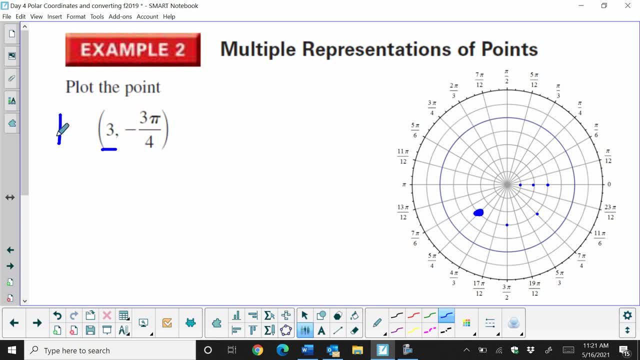 is the point, And we'll call that A. Now, point A has different representations. I can now write that with a positive radius, But this time I'm going to rotate in the positive or the counterclockwise direction, So that's just going to be out 3 and then rotate. That's 5 pi fourths. So there's a second representation for that same point. 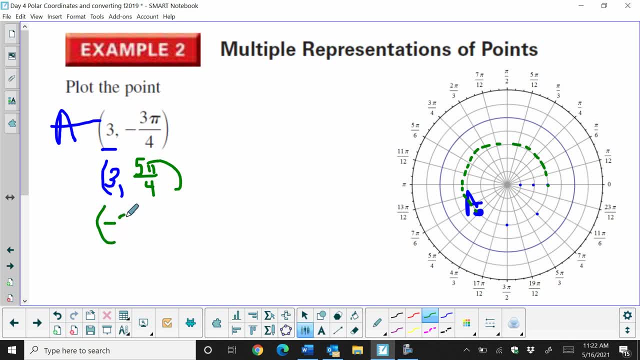 Now what if I write it with a negative radius? Well, I can write it with a negative radius, but a positive rotation. So we're going to go over 1,, 2,, 3. And this positive rotation would be pi fourths. 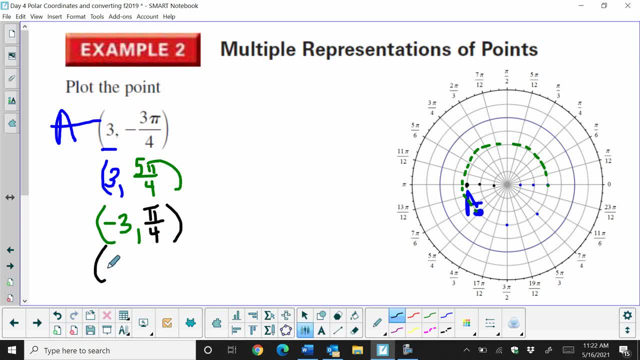 And then I can also write it with a negative radius but a negative rotation. So let's look, If I start here at negative 1,, 2,, 3, I'm going to rotate and then negative direction all the way to here, which we know as negative 7 pi-fourths.